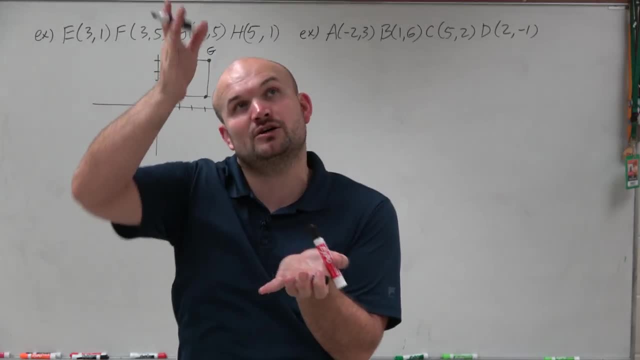 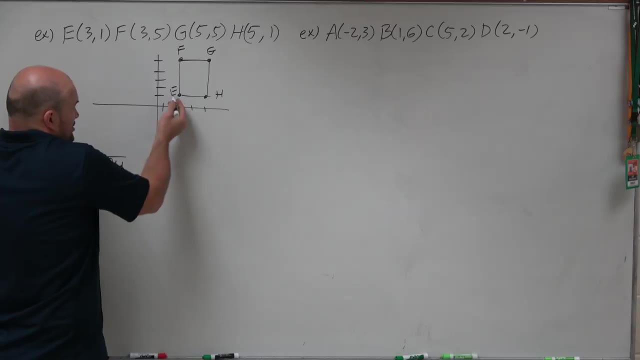 that. so the base is going to be flat and the height is going to be a measure that's going to go directly to the top. So we can see that if we were going to call, we could call EH our base, And we can really just count the difference on the base here. You can see that. 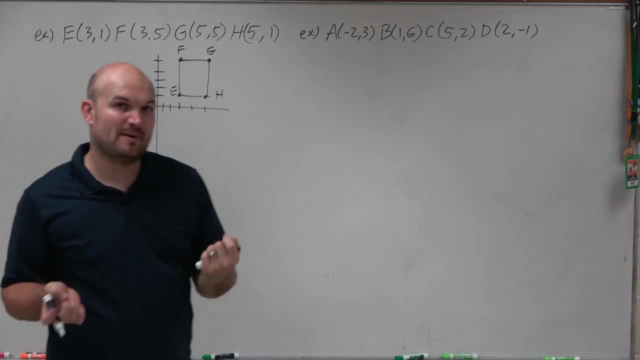 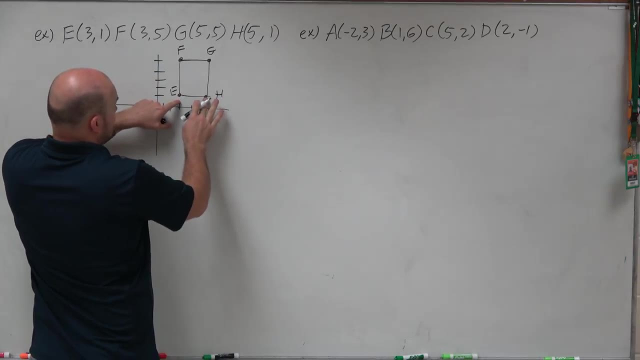 it's equal to two units. Also, we could kind of go back to our number line theory. if you remember and really look at that, The EH is the difference of our x-coordinates. So I go to E, to H and I just find the difference. 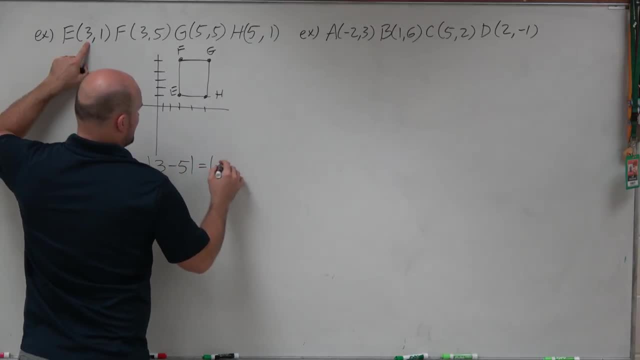 of them, Absolute value of 3 minus 5,, which is equal to negative, 2,, which is equal to 2.. However, I know, guys, it's much easier just to look at the graph and say it's 2,. 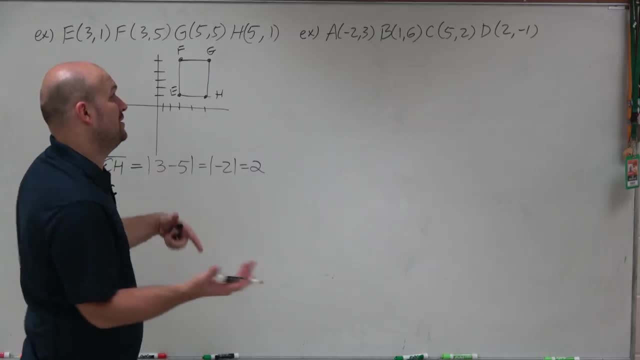 right, But I just want to go back. That was something that we learned before And I just want to say, hey, that's why it works. And then EF is going to be our height. So if we find EF, we can just count that We don't need to do the absolute value 1,, 2,, 3,, 4.. That's. 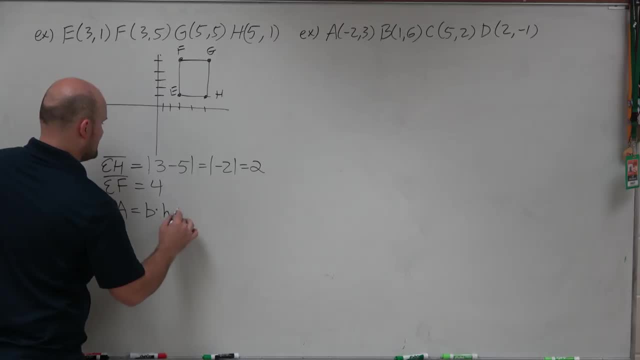 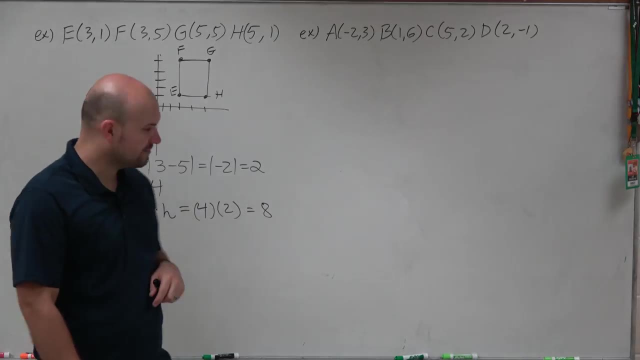 equal to 4.. So therefore, the area of a rectangle is base times height. So in that case it's going to be 4 times 2, which is equal to 8.. Now to go ahead and find the perimeter, we've got to find the distance around the rectangle. 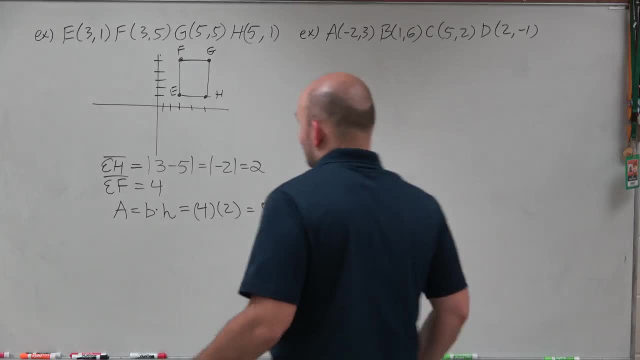 Basically, we've got to add up all the sides. Now, what's nice about this is: I know that this is a rectangle, right? I mean, it's very easy for me to say: you know that's 4.. Well, 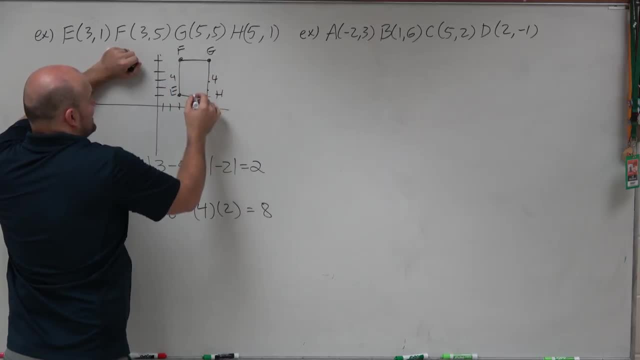 I can easily count here 1,, 2,, 3,, 4.. And then these two are 2 and 2.. So it's very easy to kind of verify that And let's just go and add them up: 4,, 8,, 10, and 12.. So perimeter. 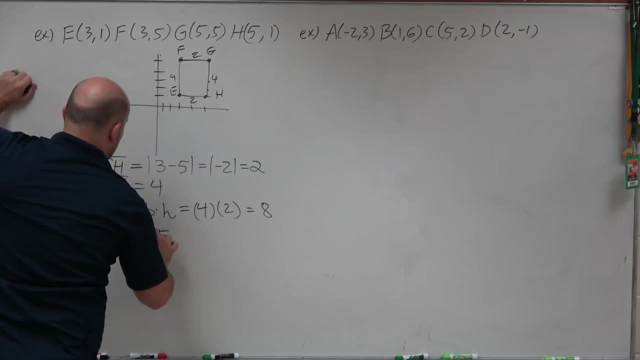 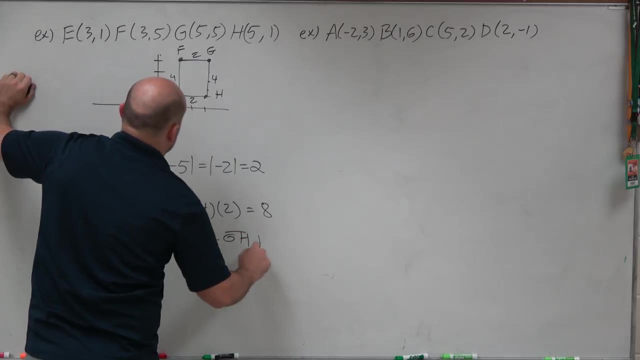 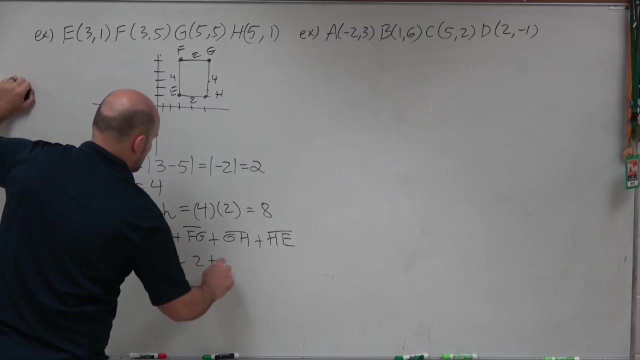 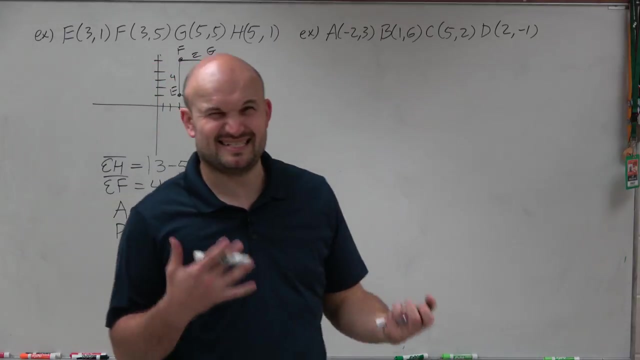 is going to equal all the side lengths. So I'm just going to write it out, just so you can kind of see: EF plus FG plus GH plus HE, So there's four sides And we're basically just adding them all up. So 4 plus 2 is 6. So that equals 12.. Just so you can kind of see it kind of written. 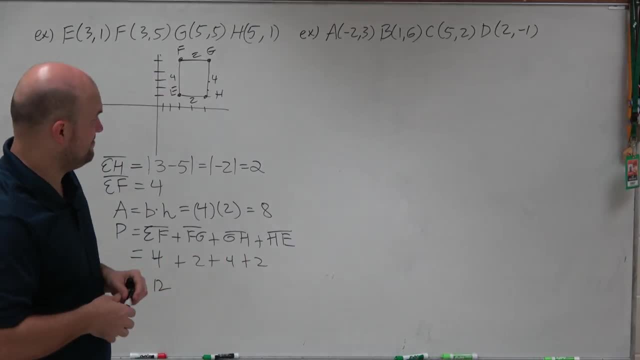 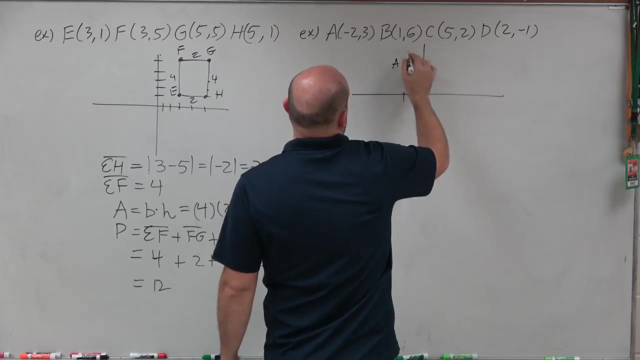 out there All right, So let's move on to the next one. We have the points A, B, C and D, So let's go ahead and plot them up. A is at negative 2, 1, 2, 3.. B is at 1, 6.. 1, 1, 2,, 3, 4, 5,. 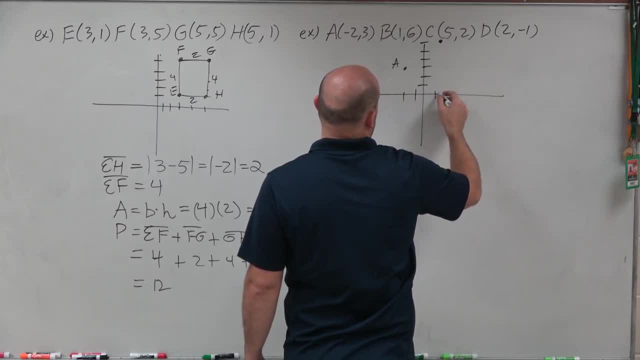 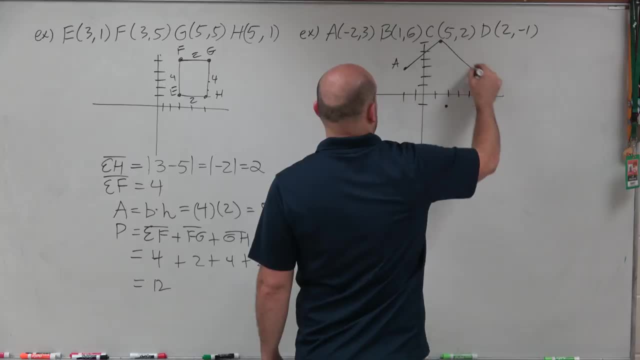 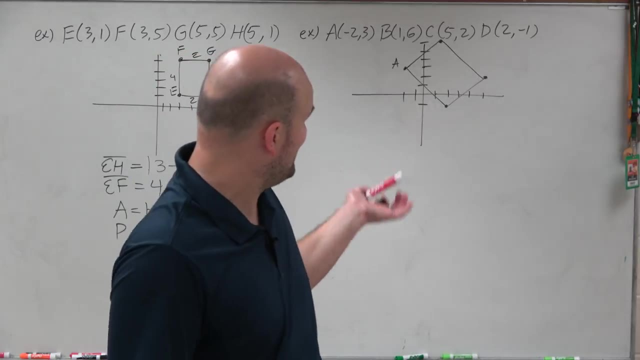 is at 2,, 3,, 4,, 5,, 6.. And D is at 1,, 2,, 3,, 4,, 5, 6.. OK, Now you got to be careful, especially when you're graphing this, because for me it looks like a rectangle, But it kind of. 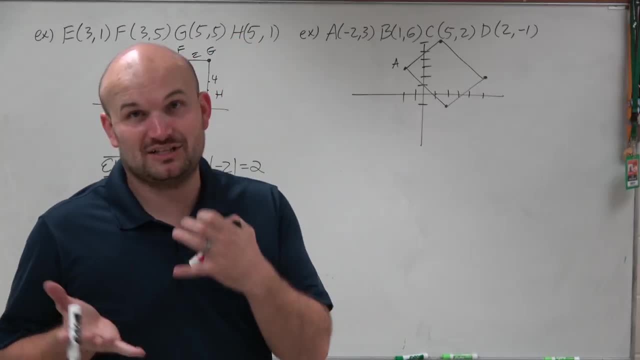 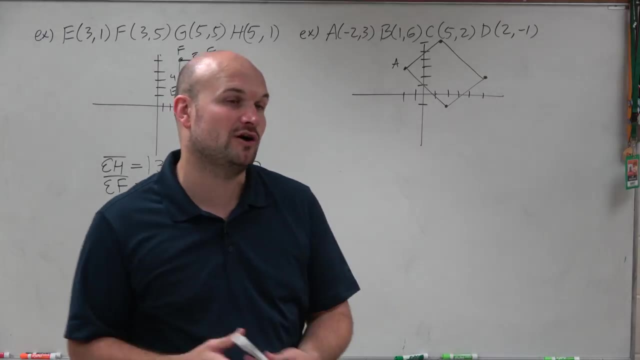 looks a little tilted. I'm not very, very sure if I'm exactly dealing with a rectangle or not. So what we want to do is we want to use the distance formula to be able to confirm. Now I'm going to do the distance formula for two sides And then I'm going to do the Pythagorean. 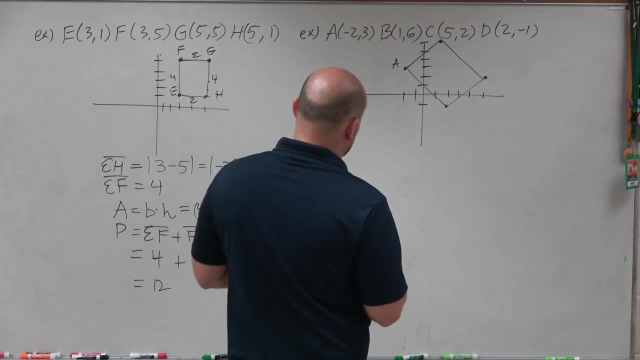 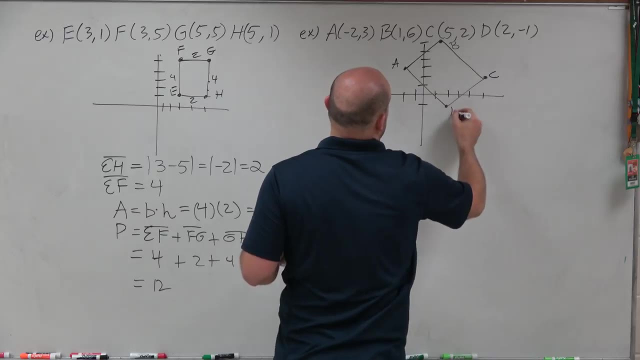 theorem for the other two sides. So let's go ahead and figure out, Let's do the distance formula, distance formula first, and let's- I forgot to label these- that's B, this is C and that's D. So let's go ahead and find. remember the distance formula is equal to X2 minus X1. 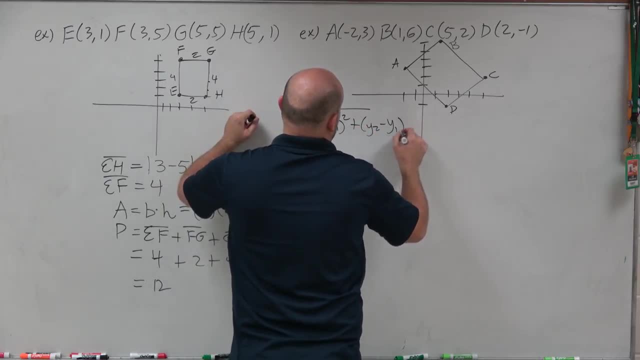 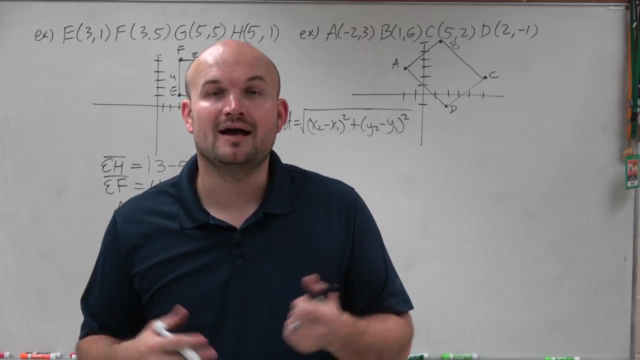 squared plus Y2, minus Y1.. So whenever you're given two points, you're basically or two points, you're basically just going to label them X and Y's with subscripts- either one or two, and then you're finding the distance and squaring them, which is basically the 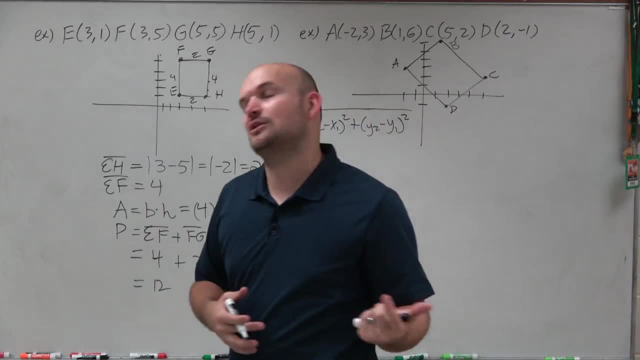 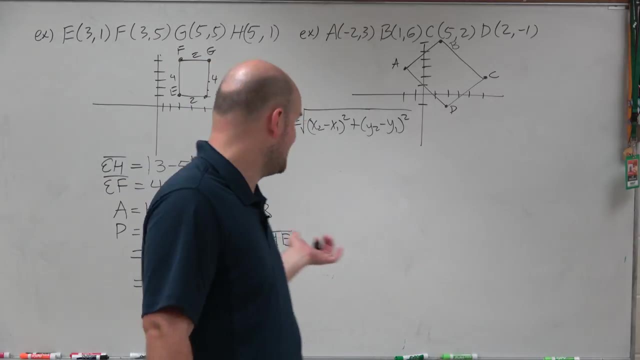 Pythagorean theorem, which I'll be able to show you and verify when I do the other points. But for right now let's just kind of say: all right, here's your, you know, let's, here is your basic formula. let's just kind of use the formula and then we'll kind of show. 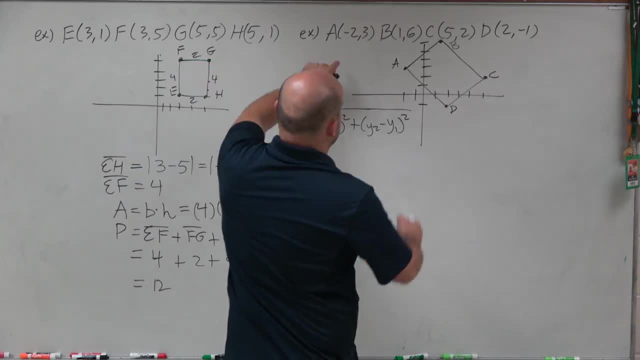 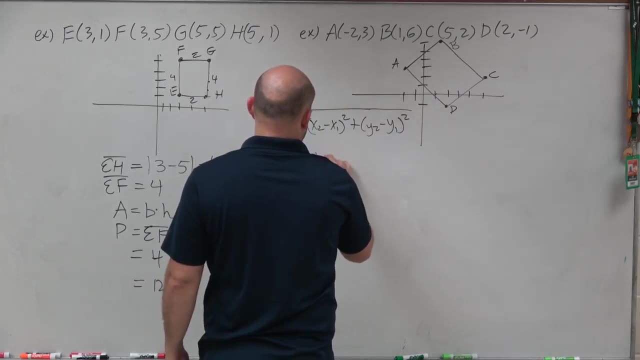 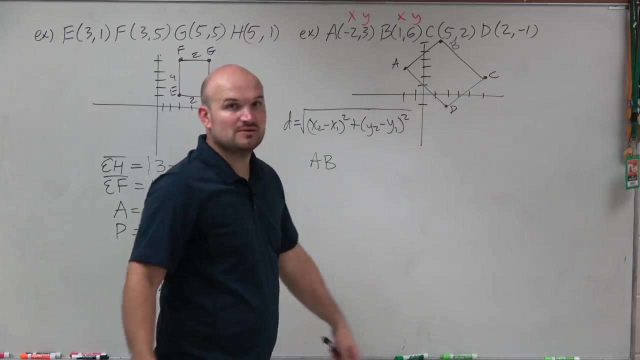 again the relationship with the Pythagorean theorem. So let's figure out AB, let's do AB and AD, let's find these two links. So if I want to find AB, basically what I'm going to do is I'm going to label my points as X and Y's right, because they're both X and 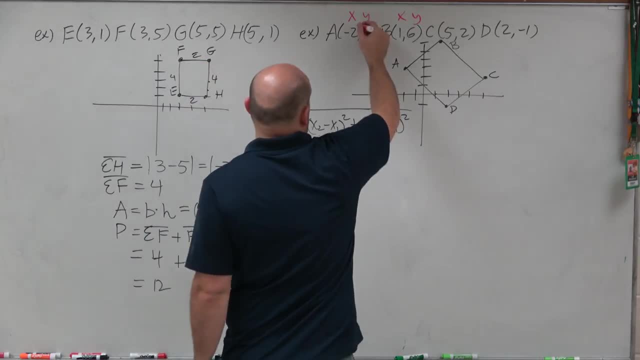 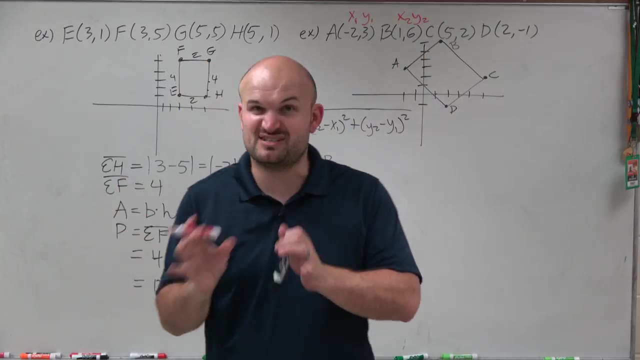 Y's. but to differentiate between which X I'm talking about, I'm going to say this is X1 and that's X2.. And then I'm going to say that's Y1 and that's Y2.. So just make sure you keep the 1's and the 2's together. 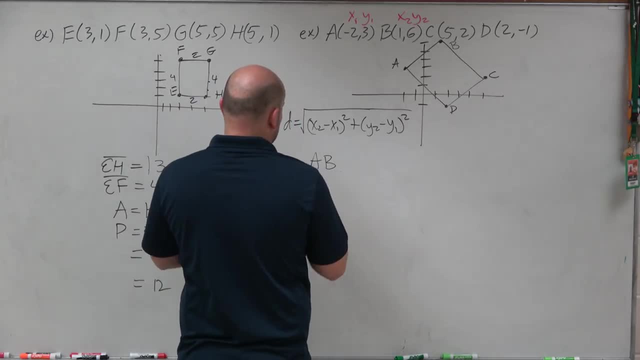 as far as X and Y's goes, Then all I'm simply going to do to find the distance, because distance of A distance is equal to AB- all I'm going to do is just plug those values into my formula. So I'm going to have X2, I don't want that there anymore, So I'll have 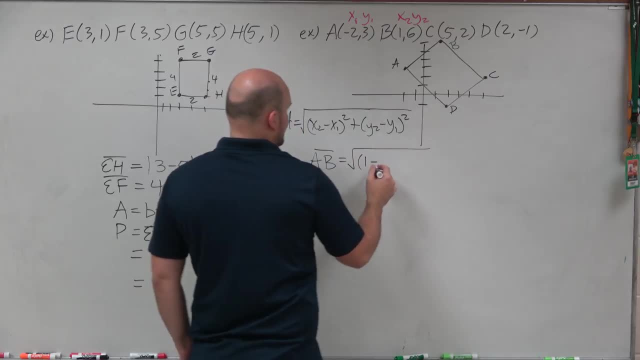 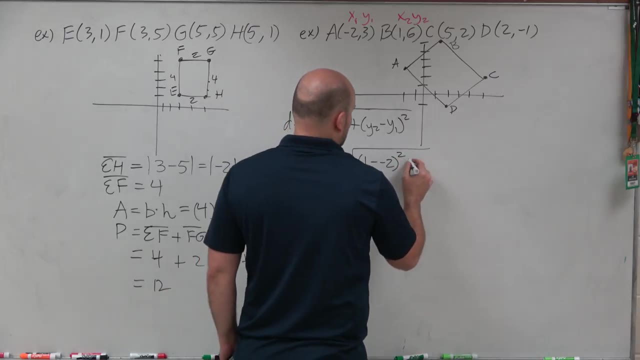 X2, which is 1 minus AB Negative 2.. Now make sure you plug that in 1 minus negative 2.. A lot of people will drop off the negative thinking. it's already like there, So just make sure you keep that And. 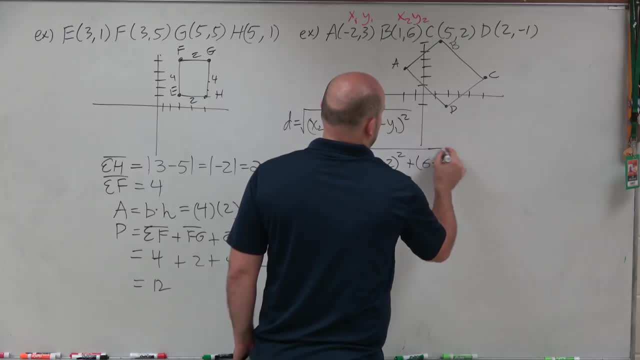 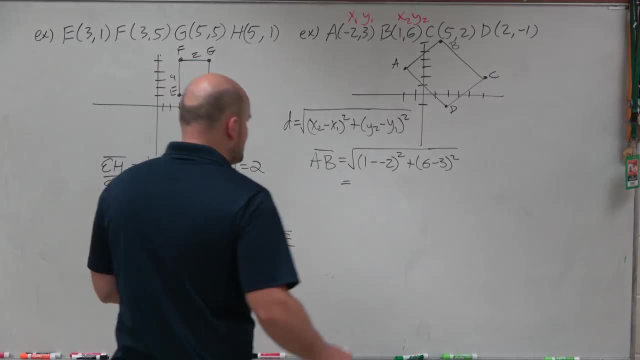 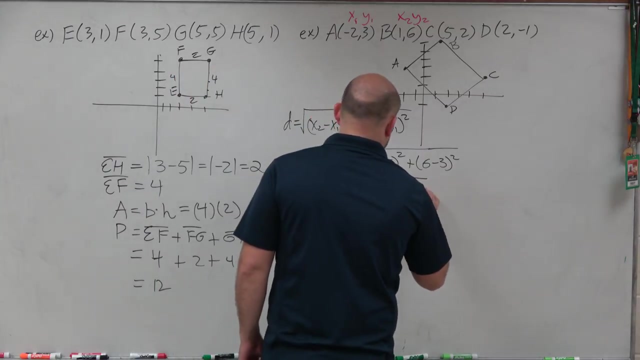 then I have Y2, which is 6 minus 3 squared. And now let's go and simplify it. Well, 1 minus the negative number is really like adding, so that goes 3.. 3 squared is going to equal to 9.. And then 6 minus 3 is 3.. 3 squared is again equal to 9.. So therefore I'm equal to. 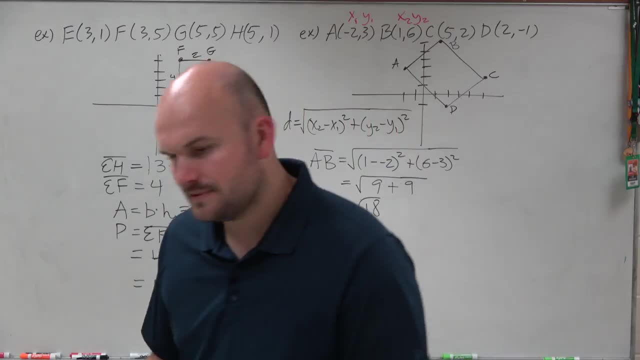 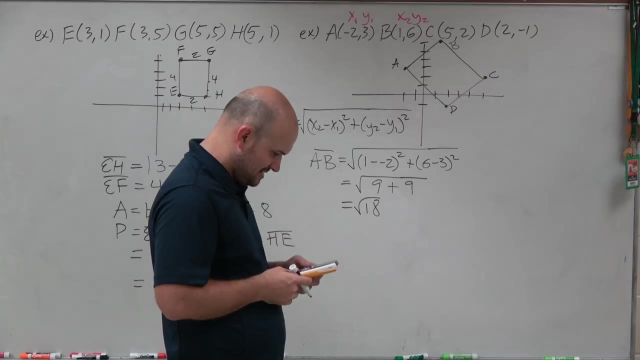 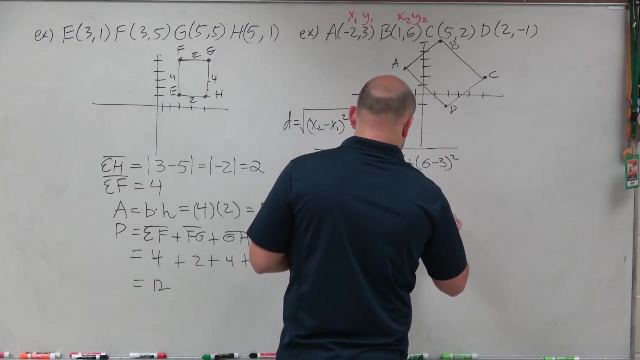 the square root of 18.. Now, dealing with the square root of 18,, I want to approximate that. So I'm going to do square root of 18, and I'm going to round to the nearest tenth, which is 4.2.. So therefore, 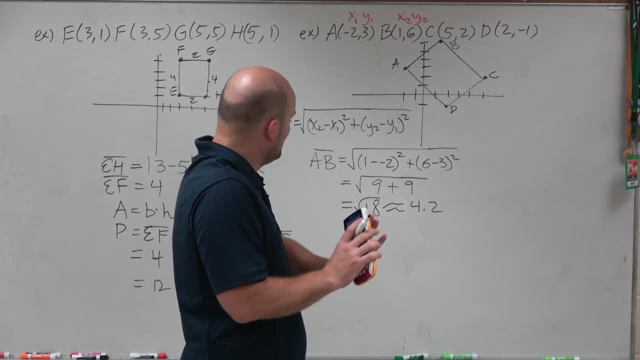 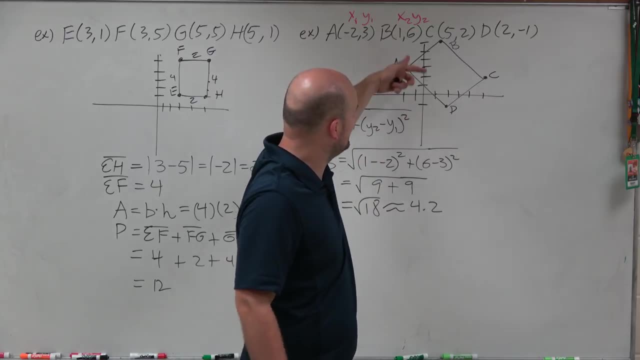 we're dealing with that at 4.2.. Now, that's actually very important. I can actually stop here for a second and verify. Well, if I know- actually I don't know- this distance height, right, I got to find that distance because I got to orientate. 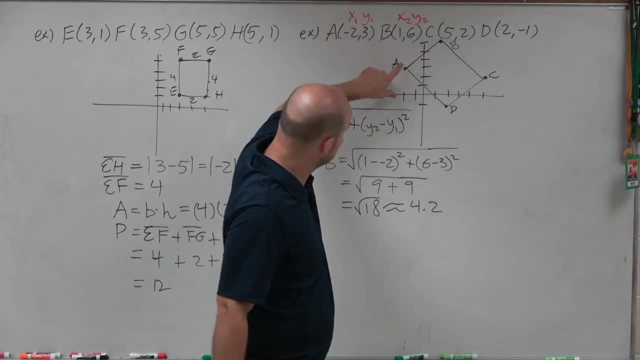 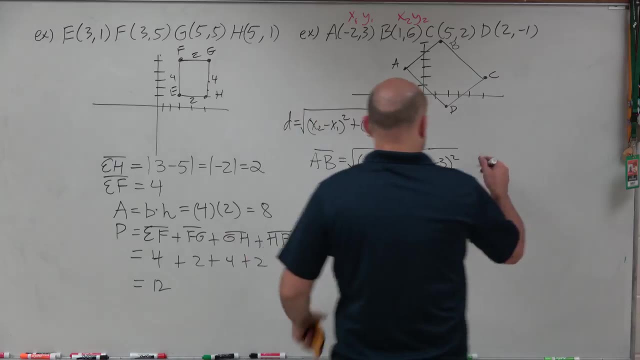 orientate this triangle. so I have one base And I'm going to call AB my base. Therefore, the height is always going to be perpendicular to your base. So therefore, I need to find the length of my AD. So let's go ahead and find AD. 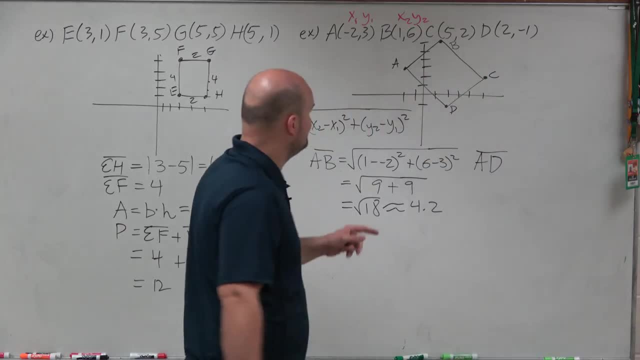 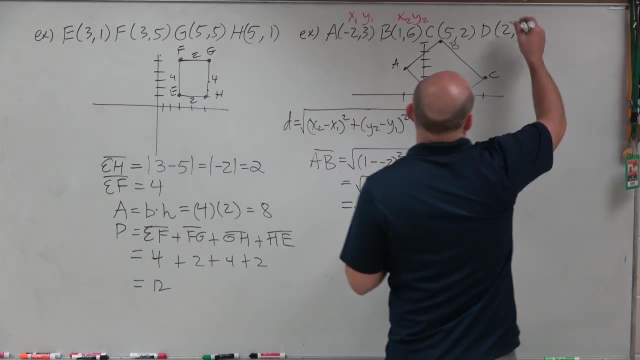 And let's do the exact same thing, except instead of calling B X2, Y2,, I'm going to now call D X2, Y2.. And you could do them X3, Y3.. I mean, it doesn't really matter. 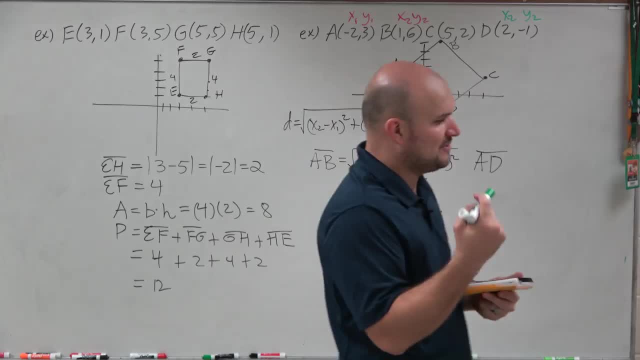 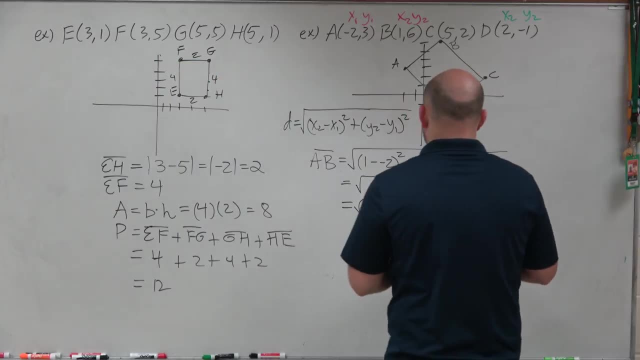 4,, 5,. it doesn't really matter what numbers you want to assign to them, It's just very important that you make sure that you distinguish which is which. So again, I'm just going to plug them now. same thing. 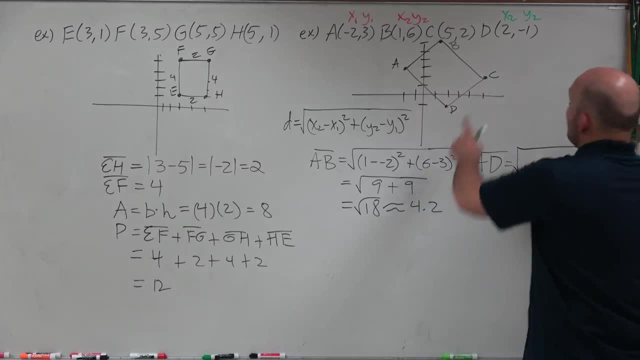 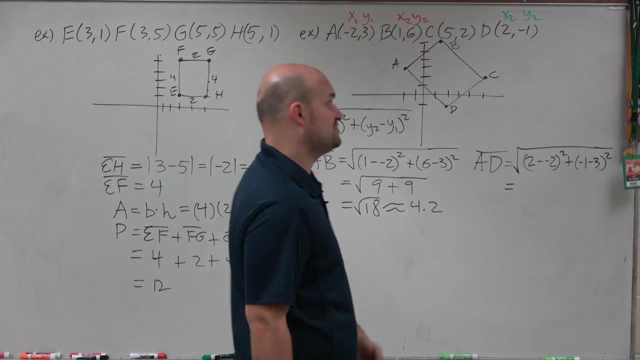 into the formula. So now my X2 is 2 minus X1,, which is negative 2, plus my Y2, which is now negative 1, minus Y1, which is 3.. So 2 minus negative 2 is 4.. 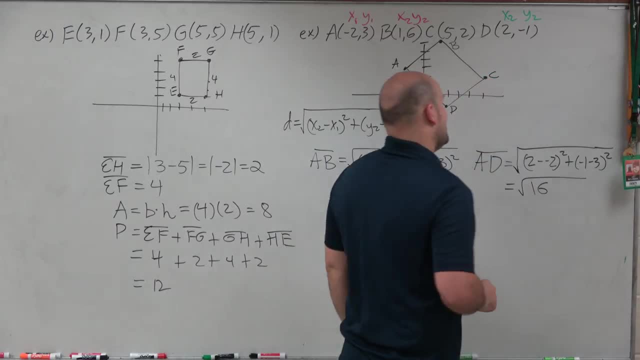 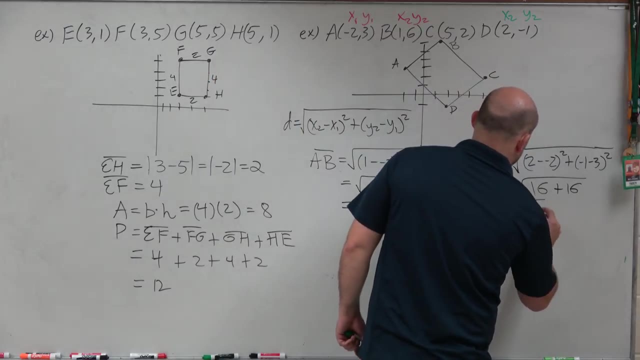 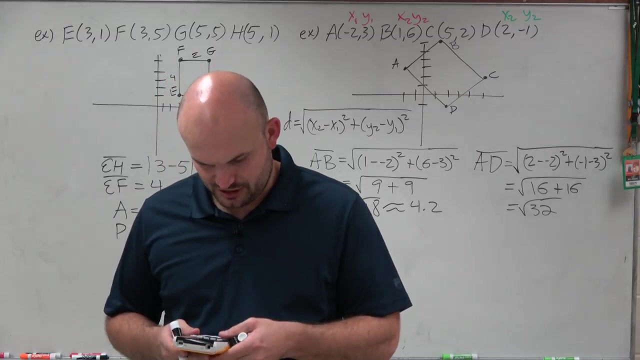 4 squared: 4 squared is 16.. Negative: 1 minus 3 is negative 4.. Negative 4 squared is also 16, which equals the square root of 32.. And then all I'm simply going to do here is just take the square root of 32 to approximate that. 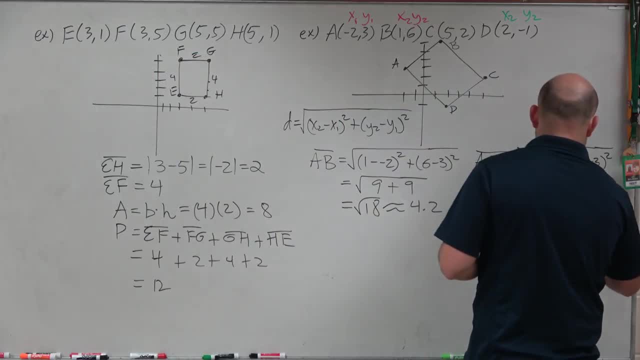 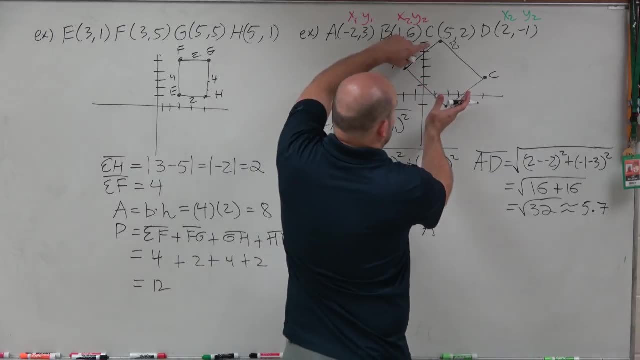 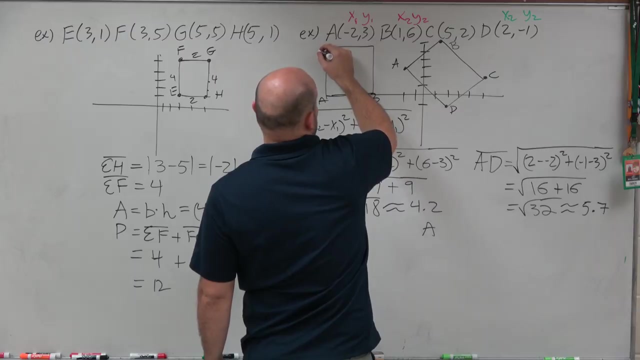 And I'm getting 5.7 is my approximation. So to find the area, if you notice, here again, if we were just to rotate this so it looked like that there's AB and there's C and D, you could see that AB is my base and AD is my height. 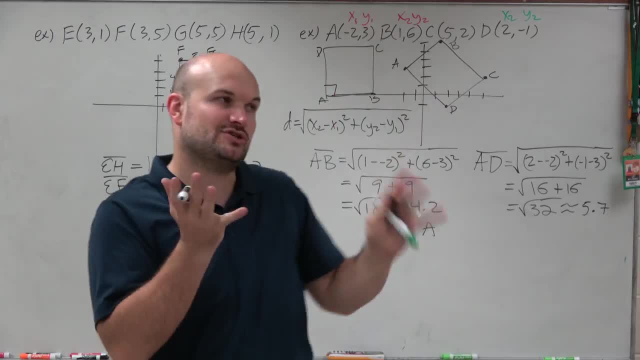 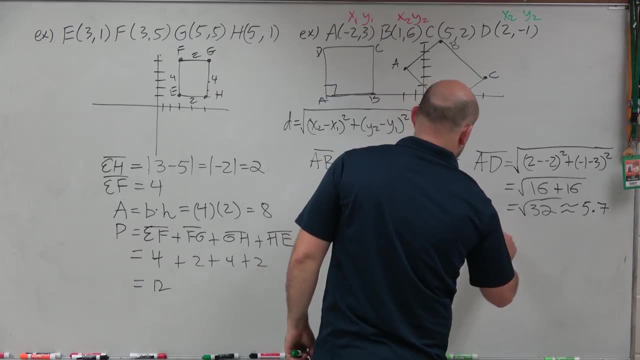 So all I'm doing is turning. I'm not changing the size of the rectangle, All I'm doing is turning it. So, therefore, AB is my new base, which is 4.2 times 5.7.. And that is going to be equal to. 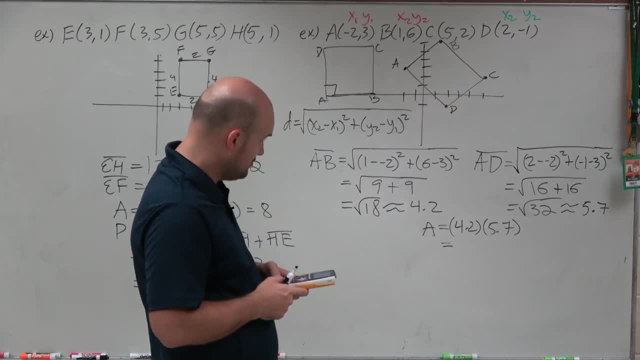 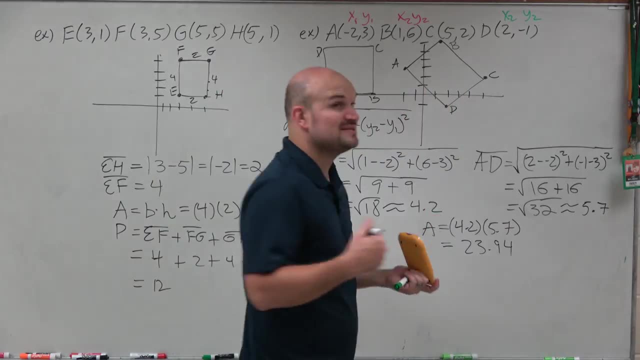 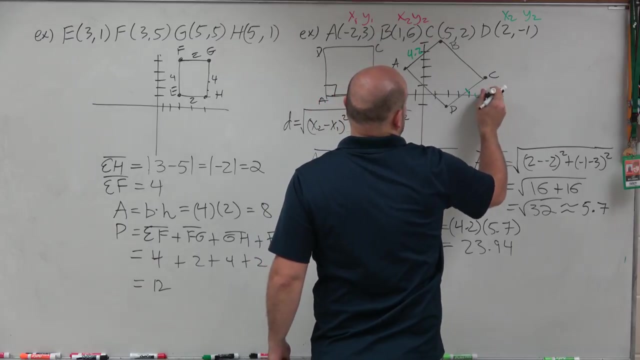 2. 4.2 times 5.7.. 23.94.. Now if the problem says it's a rectangle, you can assume that the opposite sides are exactly the same. So if I say this is 4.2, then I know that that's 4.2.. 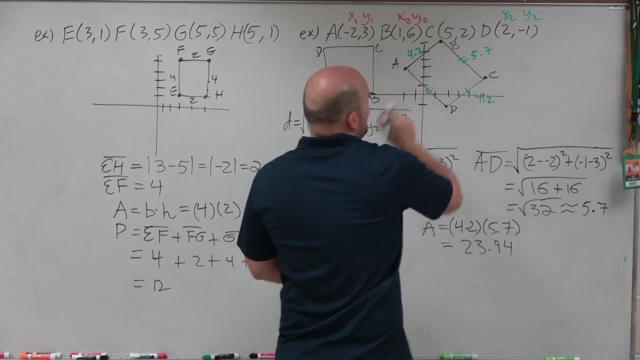 If this side length is 5.7, then I know that side length is 5.7.. But that's only if the problem says it's a rectangle. We're not sure if it's a rectangle, or at least in this video I'm not. 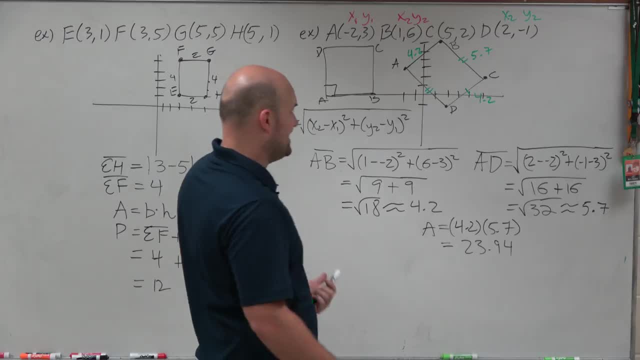 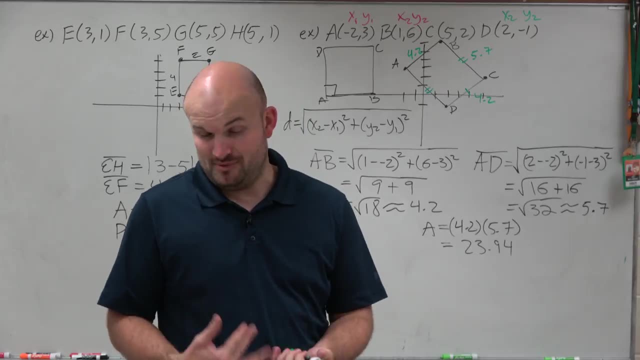 going to say that we know, We know for sure it's a rectangle. So the best bet is to verify this Now. you could do the distance formula again, Or what I kind of prefer is just using the Pythagorean theorem. And the way that I use the Pythagorean theorem. 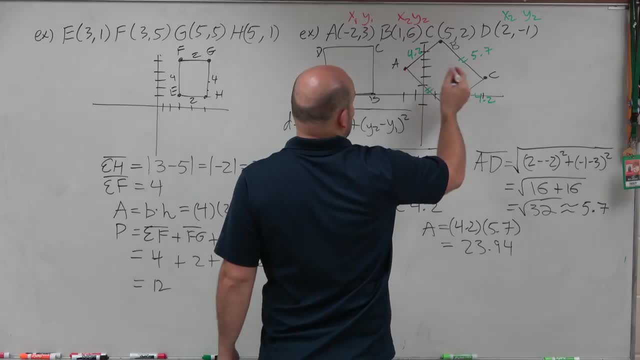 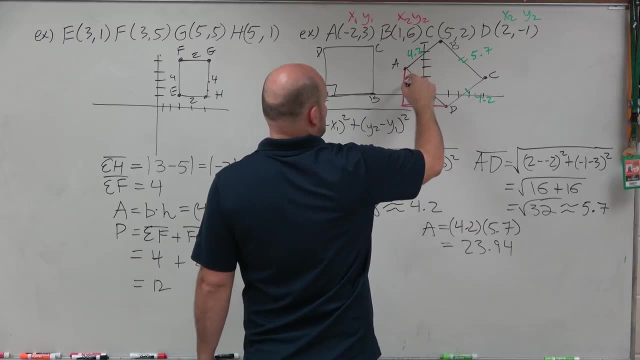 is to create right triangles. So basically to find AD, just create a right triangle. How far is this distance? I can easily count One, two, three, four. How far is this distance? One, two, three, four. 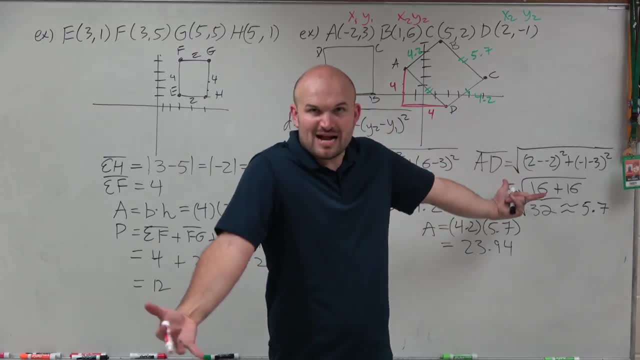 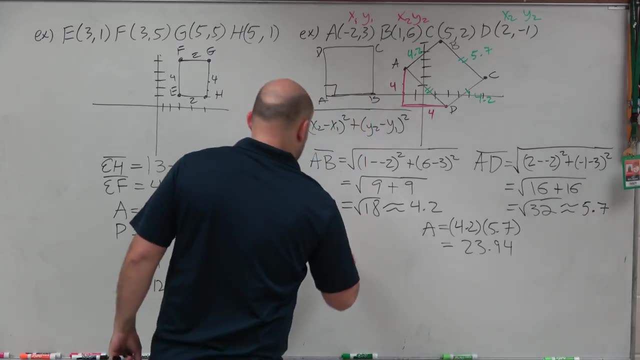 Right, And that's basically what I did over here When I was doing AD. I was subtracting them right And you see I got 4 and 4. And each time I squared them, I got 16.. So therefore, when finding AD, AD is equal to the same thing. 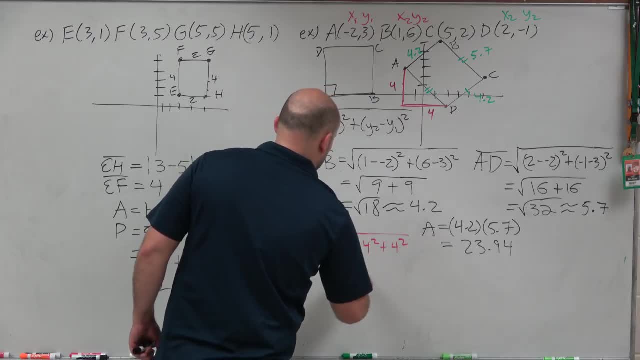 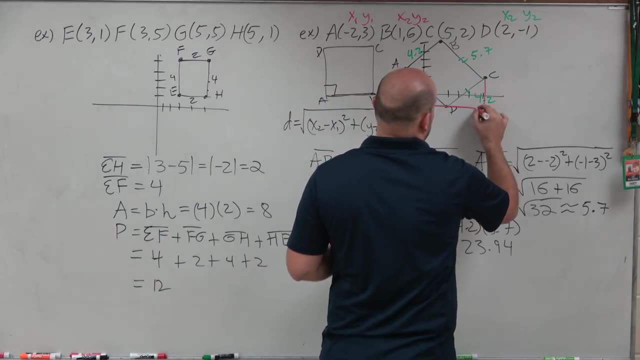 It's 4 squared plus 4 squared, which is equal to square root of 32, which again is going to be 5.7.. Now let's do the same thing over here. Over here, this distance from D to C is 1,, 2, 3.. 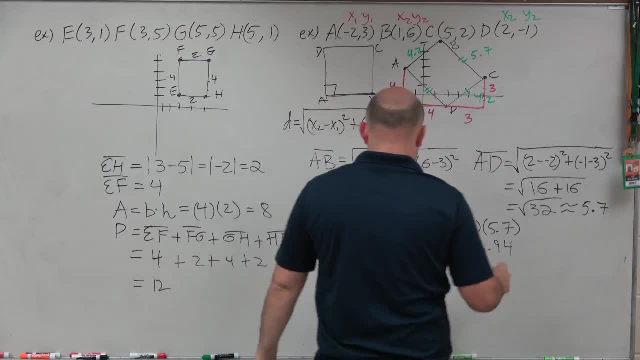 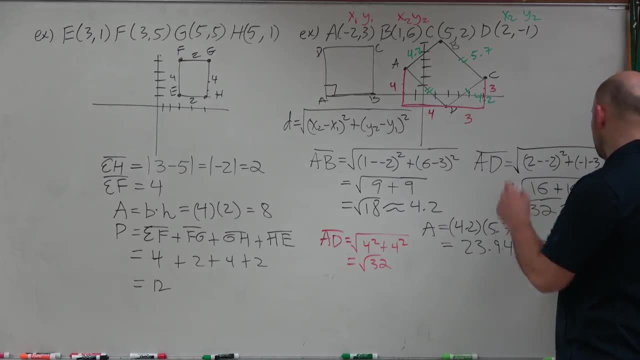 And this distance is 1,, 2, 3.. So, therefore, if I want to see DC using the Pythagorean theorem, that's going to be the square root of 3 squared plus 3 squared, which is the same thing what I had here, which is 9 plus 9.. 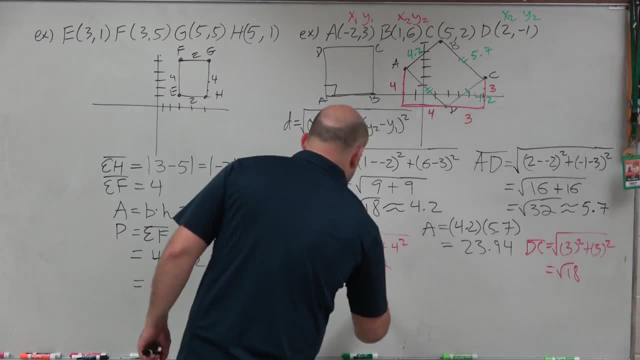 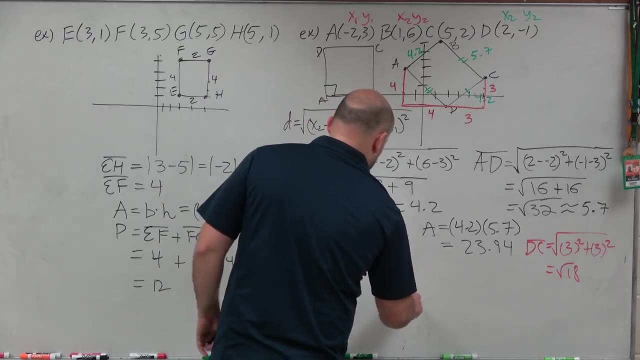 So, therefore, that's going to equal the square root of 18.. So to find the perimeter, all I simply can do- now I've verified that it's a rectangle- all I'm going to do is do I'm going to find each side length and multiply it. 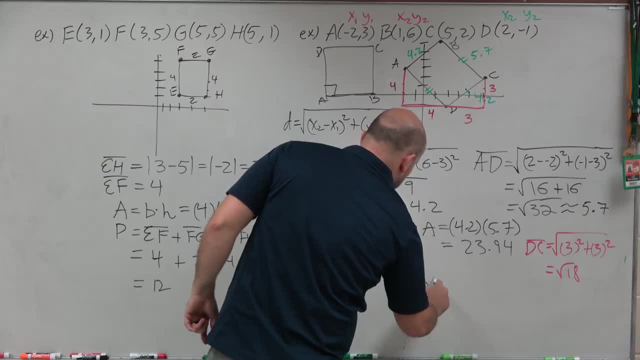 by 2.0.. Because I have two 4.2's and I have two 5.7's. So I'll do 2 times 4.2 plus 2 times 5.7.. So 2 times 4.2 is 8.4 plus 2 5.7 is 11.4.. 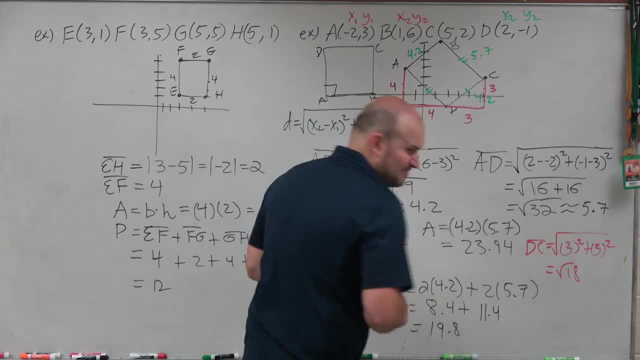 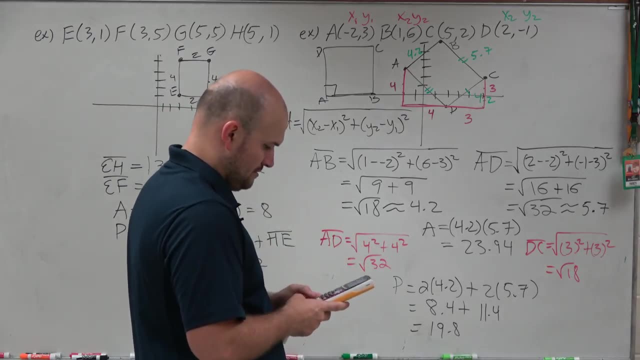 And therefore that's going to be 19.8.. But I'm going to go back in my calculator just to make sure I did all my multiplication correct: 19.8.. So there you go. Perfect. So there you go, ladies and gentlemen. 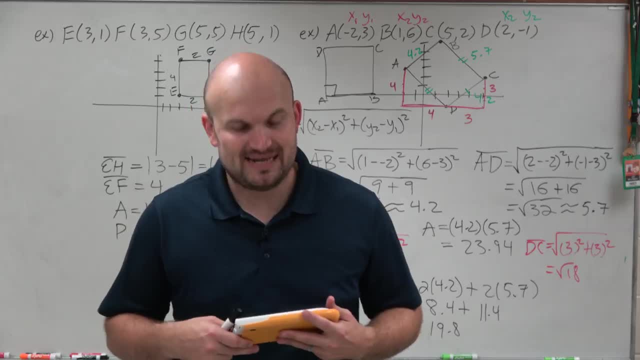 That is how you find the area as well as the perimeter, given a rectangle. Thanks,